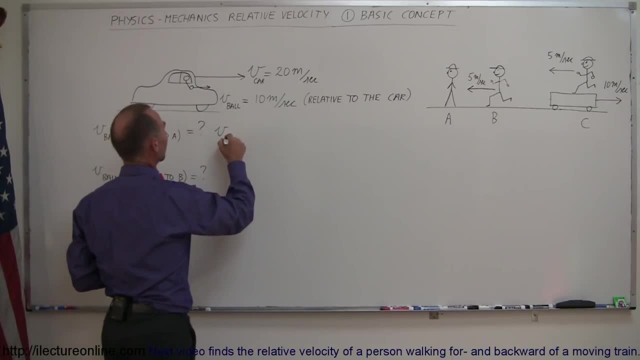 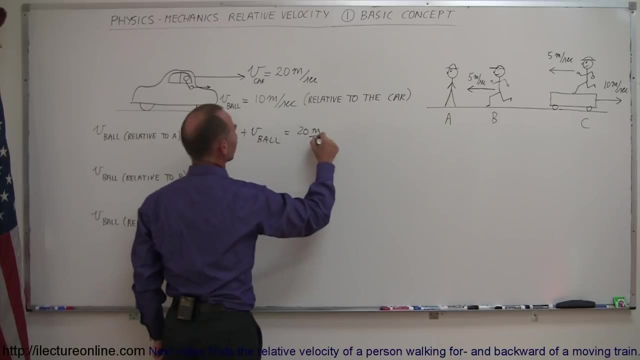 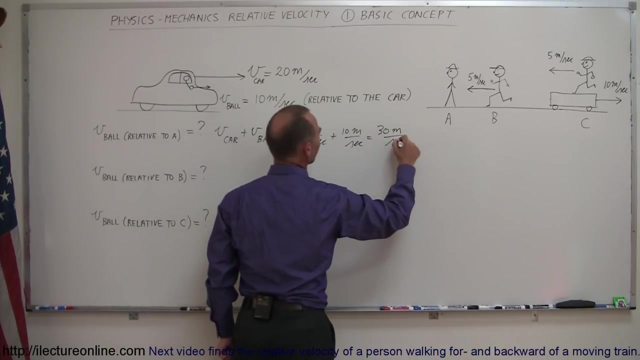 straightforward, That's going to be equal to the velocity of the car plus the velocity of the ball, And so this is going to be 20 meters per second plus 10 meters per second, which is 30 meters, And that's pretty intuitive. We can kind of look at it and say, yeah, that makes sense. 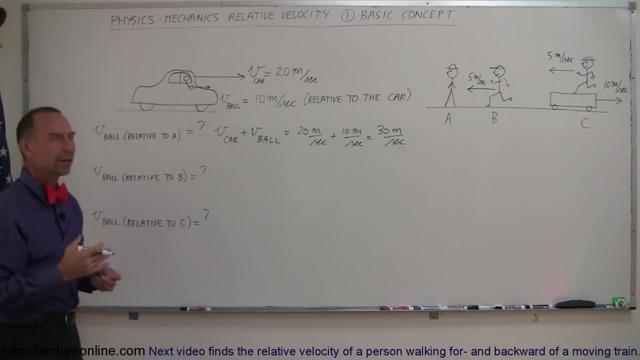 What about observer B, who's now running towards the ball? Now, intuitively, we can look at it and say: all right, that means that B is approaching the ball faster than A, So the ball should appear to be moving to B faster than to A, But B is moving to the left at five meters per second, and that. 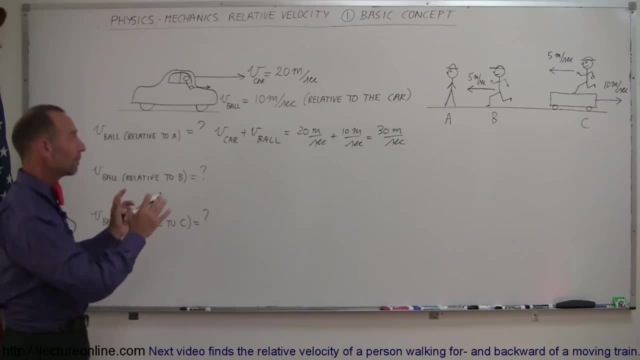 means it's a minus five meters per second. So the best way to describe it in the form of a formula is to write that B is moving to the left at five meters per second, And that means it's a minus five meters per second plus 10 meters per second, plus 10 meters per second, plus 10 meters per second. 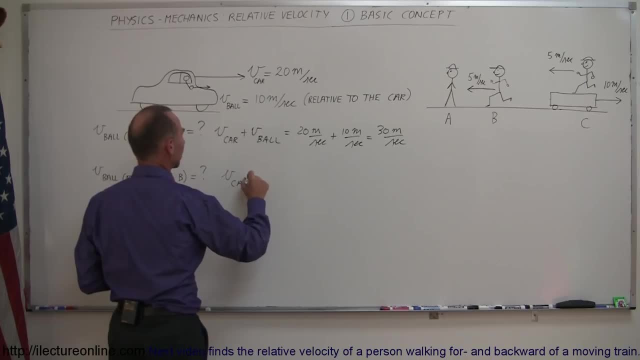 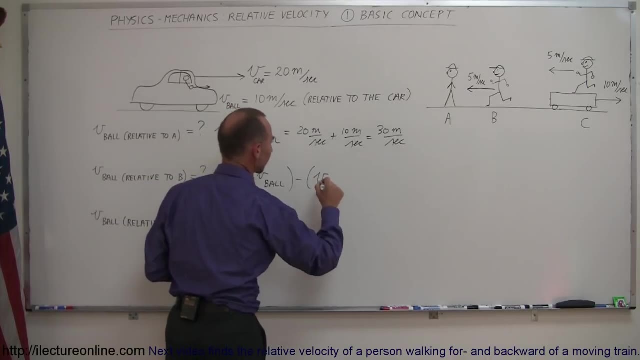 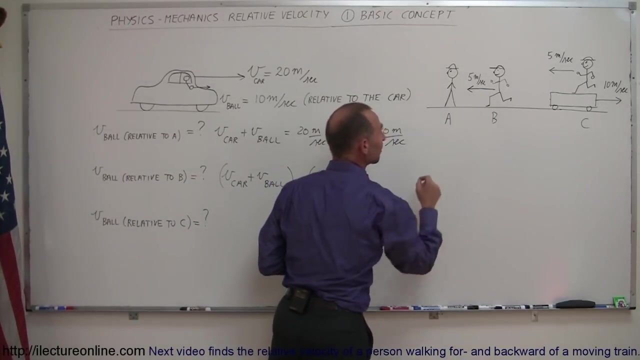 So we can write that the velocity of the ball is going to be equal to V of the car plus V of the ball and then minus V of observer B. Why we say minus? Well, it makes sense that if the observer is moving to the left at a negative five meters per second, if we subtract that, then we add that to. 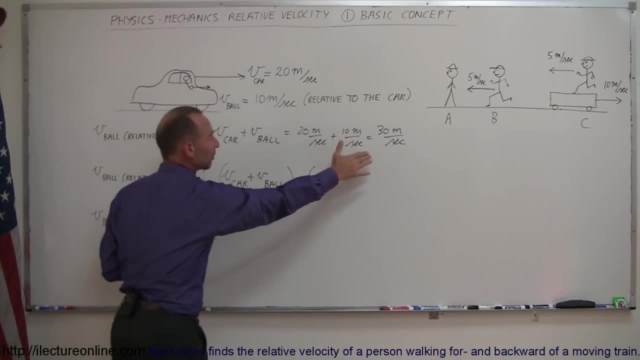 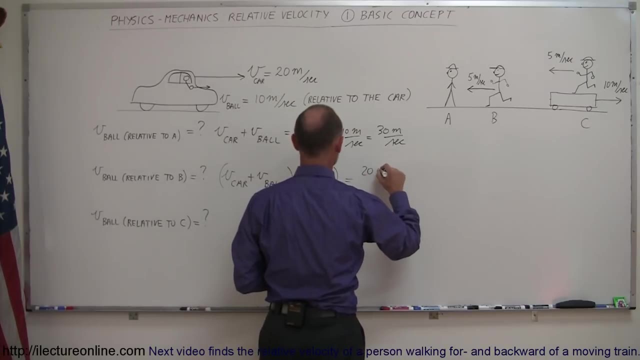 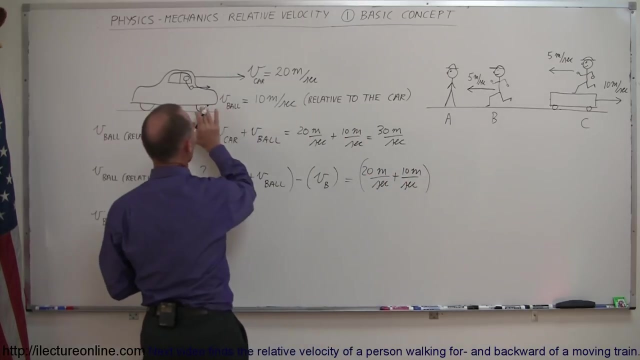 the velocity of the ball, and that means that this will then be 30 meters per second plus five meters per second, and we'll get the right answer, All right. so this then becomes 20 meters per second plus 10 meters per second. This gives us the velocity of the ball relative. 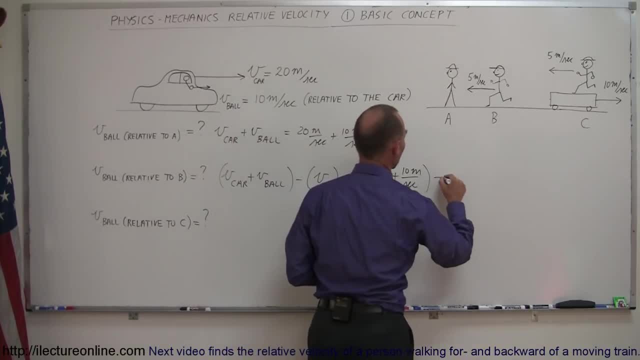 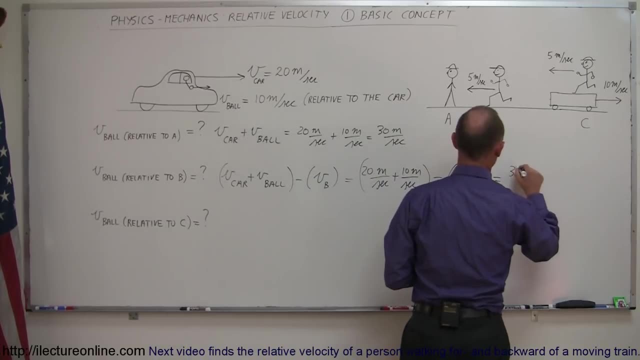 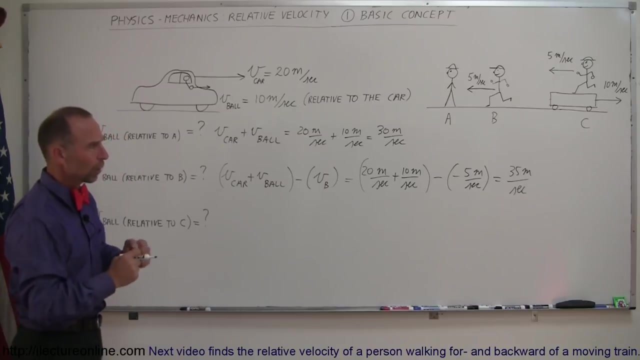 to the road or relative to the stationary observer, and that's going to be minus a minus five meters per second, which now will give us 35 meters per second. So to observer B, the ball appears to be moving faster. What about observer C, who's running on a platform that's moving to? 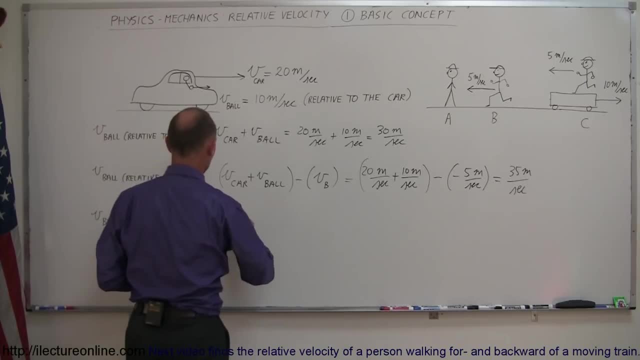 the right at 10 meters per second. All right, that will then become V of the car plus V of the ball, which again gives us the velocity of the ball relative to the road or stationary observer, minus V of the ball, plus V of the platform. 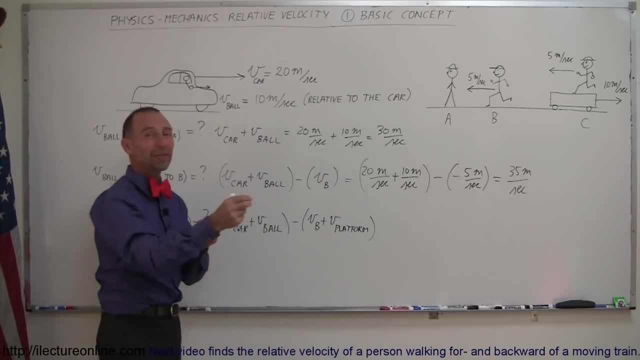 Now notice that the platform is moving to the right, moving away from the ball, so the ball has a harder time catching up. so the ball will appear to be moving slower relative to C, and so therefore we subtract that velocity and therefore we get a smaller velocity. So let's see what that ends up. 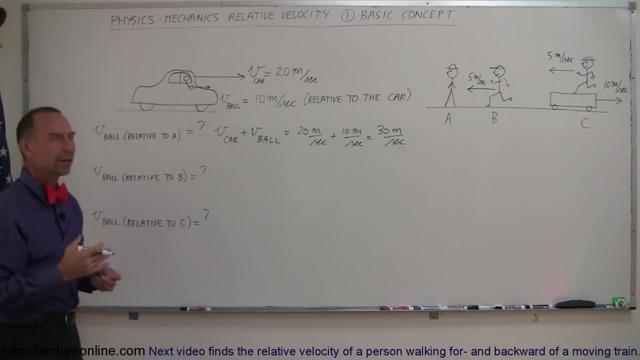 What about observer B, who's now running towards the ball? Now, intuitively, we can look at it and say: all right, that means that B is approaching the ball faster than A, So the ball should appear to be moving to B faster than to A, But B is moving to the left at five meters per second, and that. 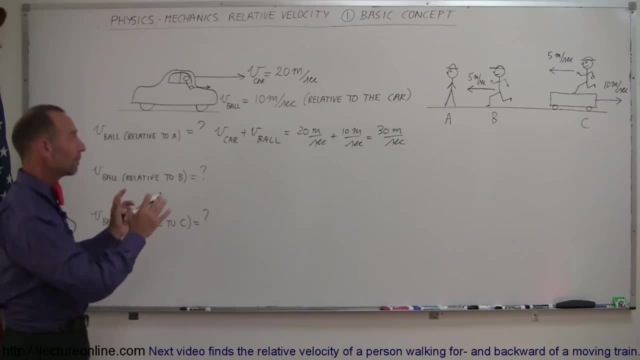 means it's a minus five meters per second. So the best way to describe it in the form of a formula is to write that B is moving to the left at five meters per second, And that means it's a minus five meters per second plus 10 meters per second, plus 10 meters per second, plus 10 meters per second. 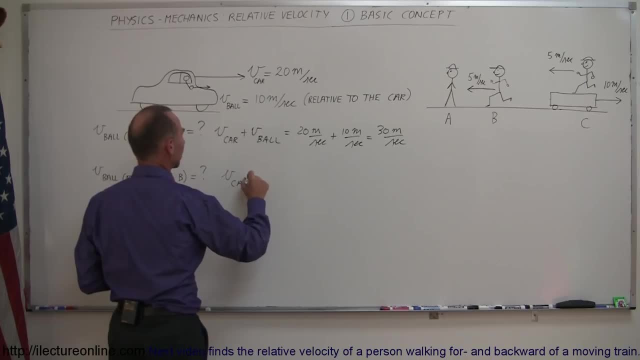 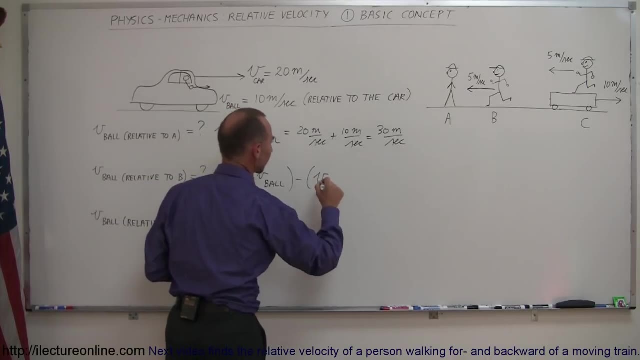 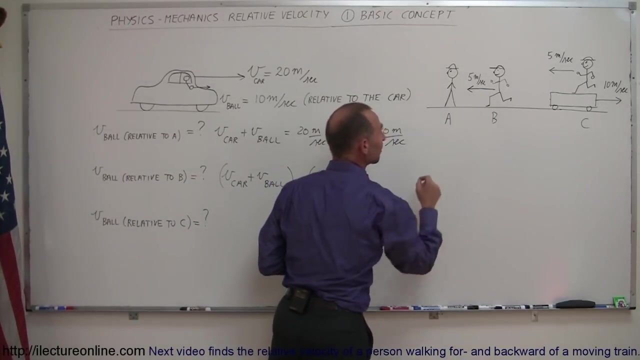 So we can write that the velocity of the ball is going to be equal to V of the car plus V of the ball and then minus V of observer B. Why we say minus? Well, it makes sense that if the observer is moving to the left at a negative five meters per second, if we subtract that, then we add that to. 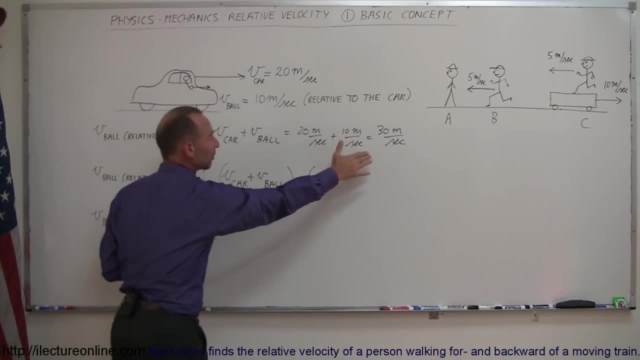 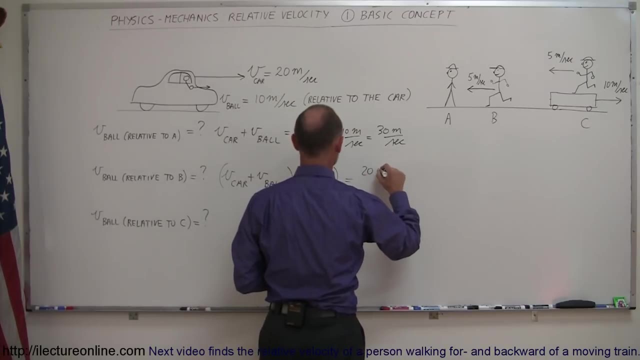 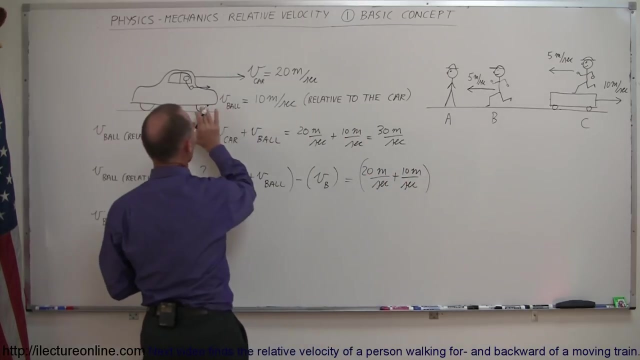 the velocity of the ball, and that means that this will then be 30 meters per second plus five meters per second, and we'll get the right answer, All right. so this then becomes 20 meters per second plus 10 meters per second. This gives us the velocity of the ball relative. 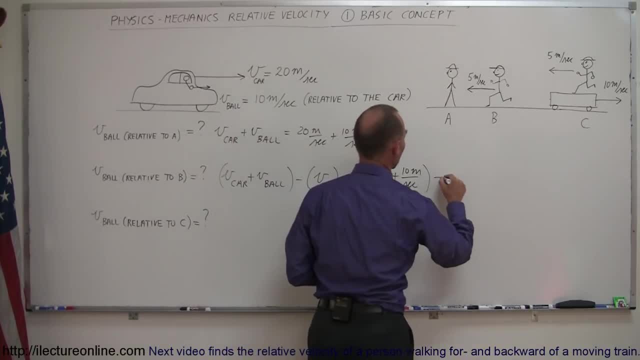 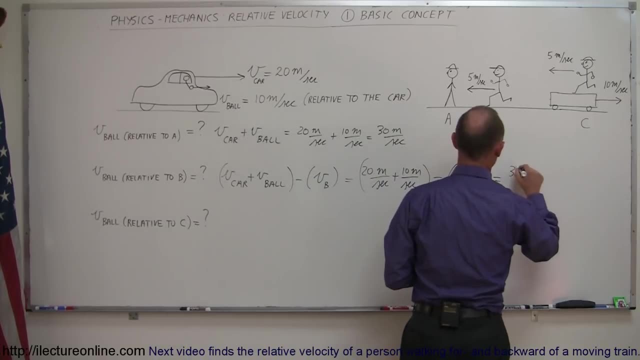 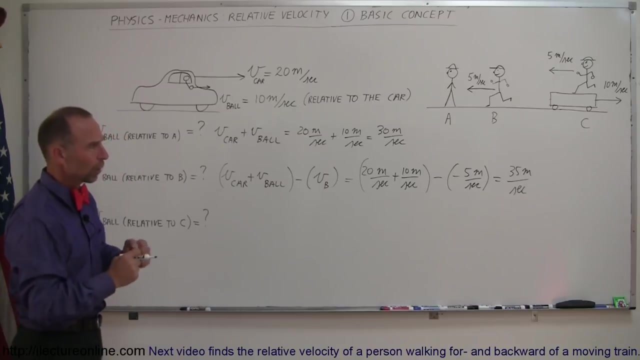 to the road or relative to the stationary observer, and that's going to be minus a minus five meters per second, which now will give us 35 meters per second. So to observer B, the ball appears to be moving faster. What about observer C, who's running on a platform that's moving to? 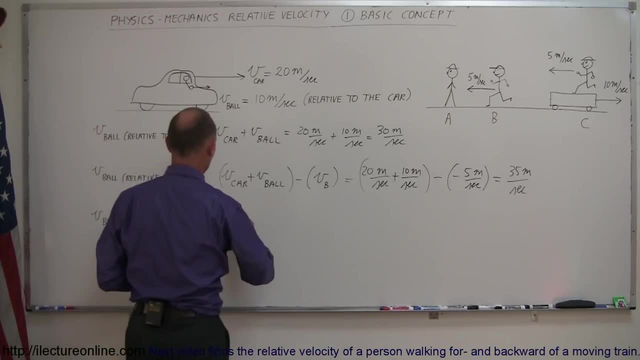 the right at 10 meters per second. All right, that will then become V of the car plus V of the ball, which again gives us the velocity of the ball relative to the road or stationary observer, minus V of the ball, plus V of the platform. 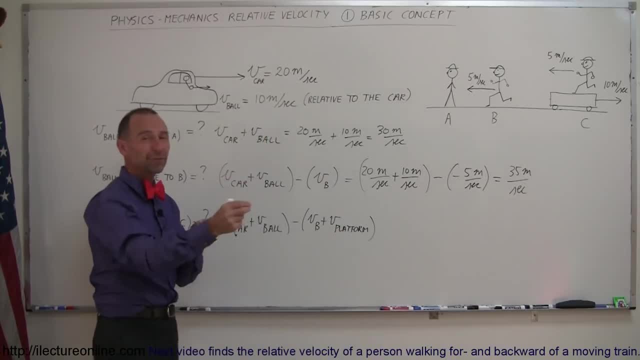 Now notice that the platform is moving to the right, moving away from the ball, so the ball has a harder time catching up. so the ball will appear to be moving slower relative to C, and so therefore we subtract that velocity and therefore we get a smaller velocity. So let's see what that ends up. 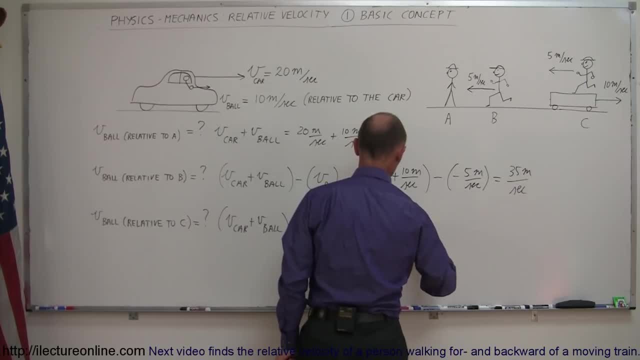 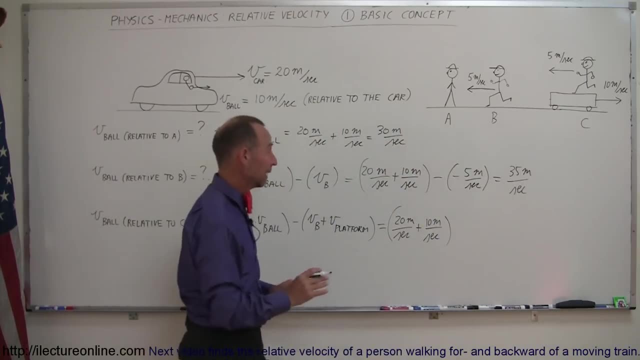 being So, this will be 20 meters per second plus 10 meters per second Again. that would be the velocity of the ball relative to the road. Now we subtract from that velocity of- oh, I should say observer C, not B, because